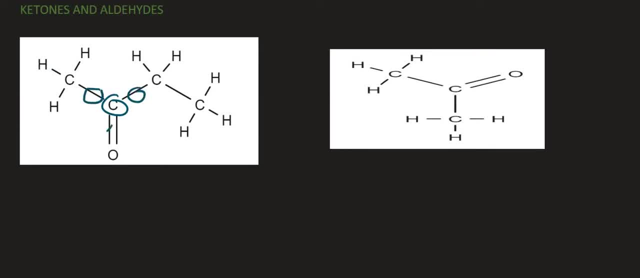 here you'd see that it's got one, two, three, four bonds, So that'll always be the case for carbon. The general formula for a ketone is the following: The number of hydrogens will always be double the number of carbons. We can see that if we look at one, two, three, four. 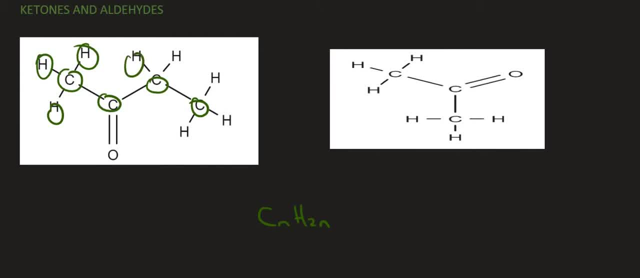 then your hydrogens are one, two, three, four, five, six, seven, eight, So that's always double, And then we've just got a random oxygen. so it will do something like that. So this is the general formula for a ketone. Now which part of this molecule makes it what it is? 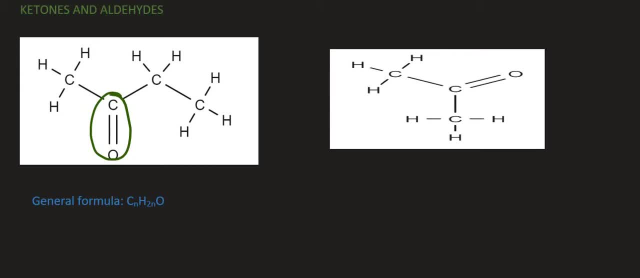 Well, it is the C double bond oxygen, but we get lots of molecules that have a C double bond oxygen, So it can't just be that. The distinguishing thing is is that that C double bond oxygen is in between two carbons, And so that whole part there that I've highlighted, that is the functional. 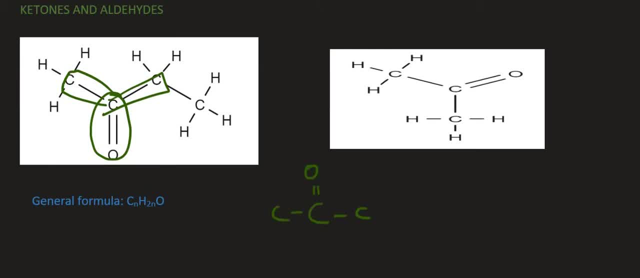 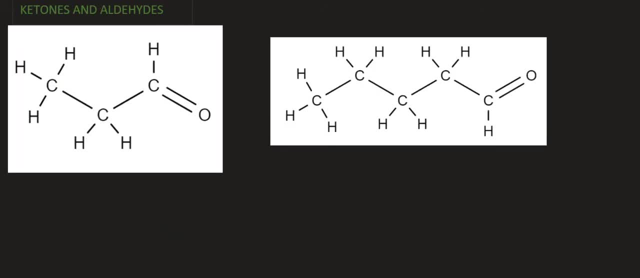 part. So it's that That is the functional group And that's it for ketones. Now we're going to look at aldehydes. Now I'm hoping from the previous videos that when you hear the word aldehyde, something in your brain is going side: Aldehyde, always on the side. So 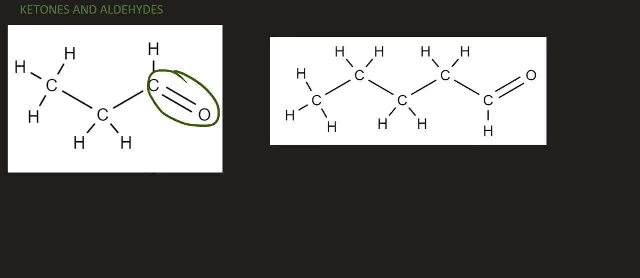 aldehydes, just like ketones, also have a C double bond oxygen. Now you see why we can't use that as the functional group for a ketone, because it's also in a aldehyde. So what makes a ketone? I mean? 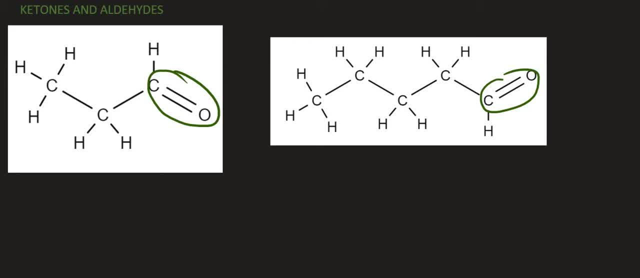 an aldehyde different to a ketone is that the C double bond oxygen takes place at the end of the molecule. So that's a C double bond oxygen And the C double bond oxygen takes place at the end of the molecule And not somewhere in the middle. So remember, your ketone does something like this, where the 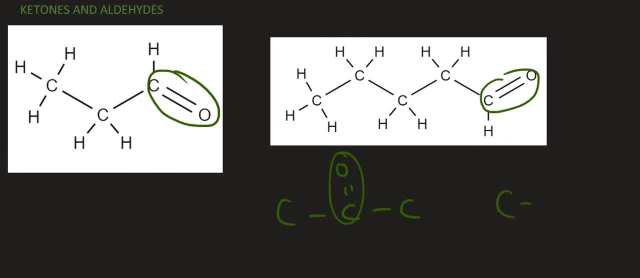 double bond oxygen is somewhere in the middle, Whereas with your aldehyde that double bond oxygen is on the side. If there was an oxygen here, then it's a typically a totally different molecule. But as long as it's just a C double bond oxygen, that's an aldehyde. So the general 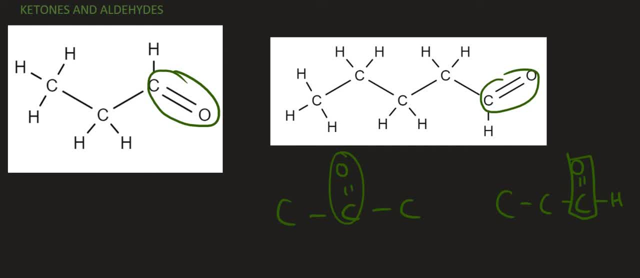 formula for this one is also going to be the same as a ketone. So that's a C- double bond oxygen- And then there's an O. So it's got the same general formula as a ketone, but they're totally different.